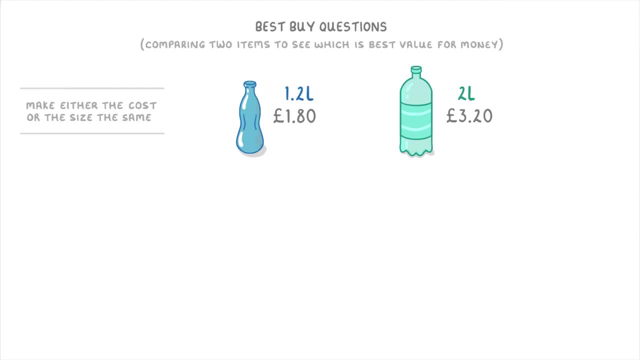 Now the other way that we could have done this question, which I think is a bit harder, is instead to find out how many litres you're getting per pound that you spend for each bottle. So, for the bigger bottle, by doing the 2 litres. 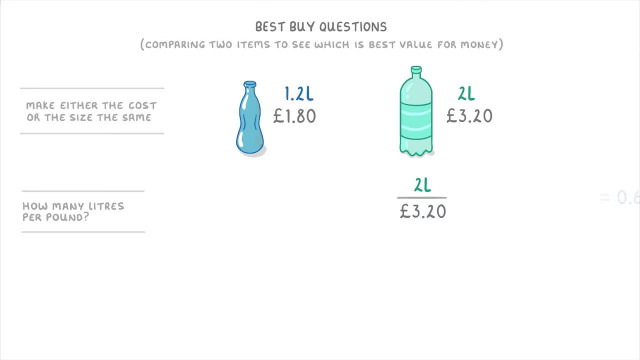 we get £1.50 per litre divided by the £3.20, we can find that we're getting 0.625 litres per pound that we're spending, Whereas for the smaller bottle we're doing 1.2 litres divided by £1.80. 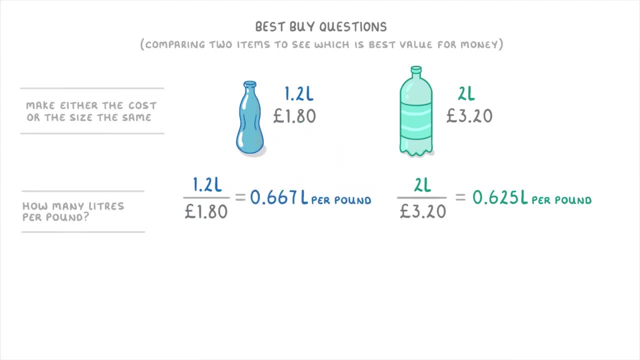 to find out that we're getting 0.667 litres per pound. So again we can see that the smaller bottle is better value because we're getting more drink per pound that we spend. If you're wondering which of these techniques are the most effective in calculating the volume of the bottles, feel free to leave a message down below to let us know. If you're interested in more details about how you can do this, visit our website at wwwsluptancomau. If you're interested in more details about how you can do this, visit our website at wwwsluptancomau. 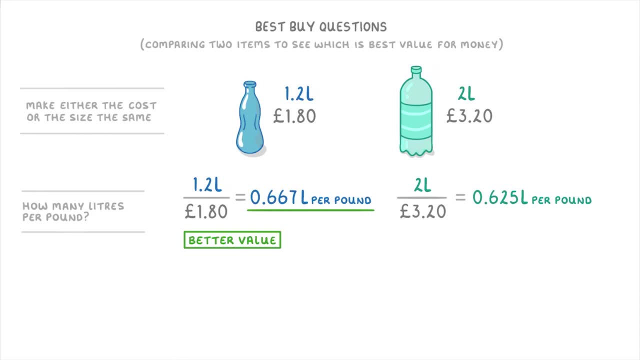 techniques you should use. There isn't really any right or wrong answer. Both are correct, But often you'll find one of them a bit easier or make a bit more sense than the other one, So just try and pick the one that fits best for you. 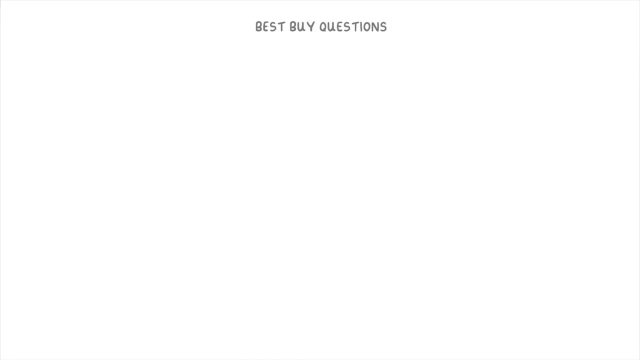 Let's have a go at one more. Imagine that we had two packs of toilet rolls: One that contains nine rolls for £4.23 and another that contains four rolls for £1.96.. And we're asked to figure out which pack is the best value. 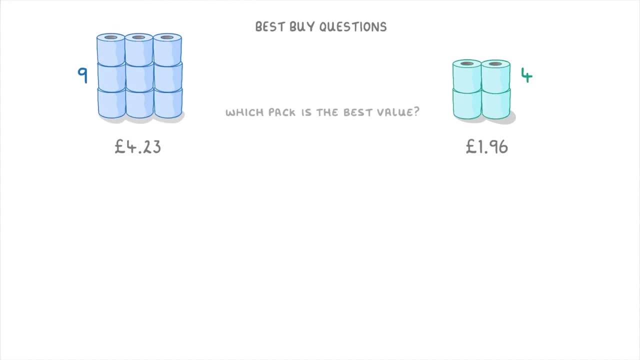 So this time it's a bit simpler to see what to do. We just need to find out how much one roll would cost in each case. So we divide £4.23 by 9 to find that each roll will cost £0.47 or 47p. 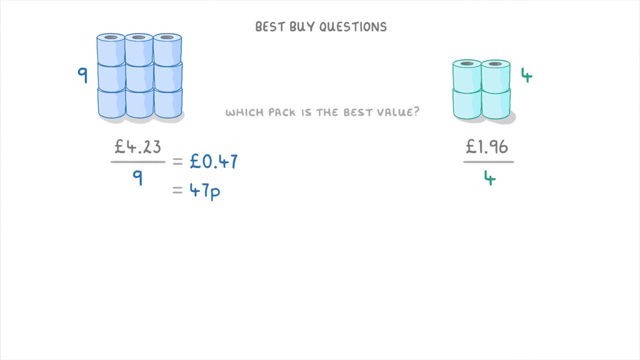 And we divide £1.96 by 4 to find that each roll from that pack will cost £0.49 or 49p. So the pack of nine is a slightly better deal because each roll costs two pence less. Anyway, that's everything for this video. So if you enjoyed it, 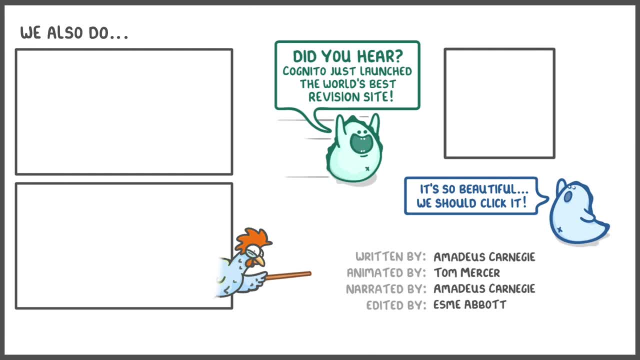 then please do give us a like and subscribe, And we'll see you again soon.